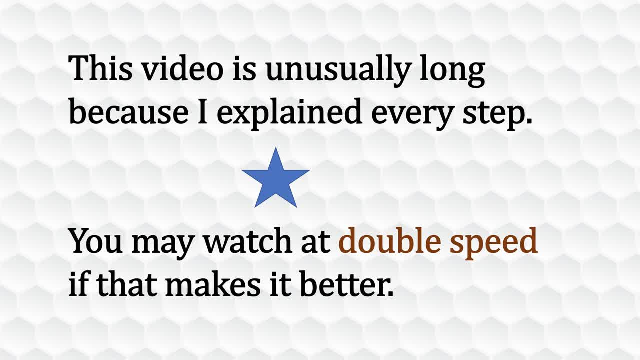 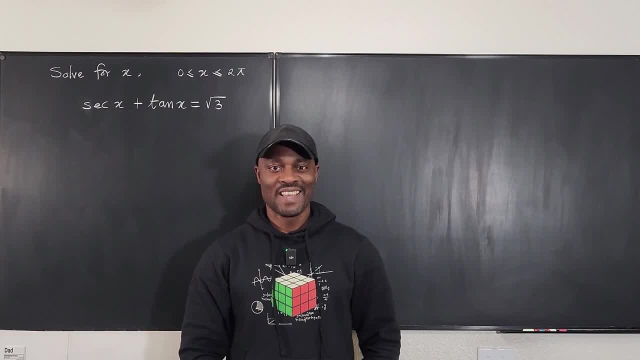 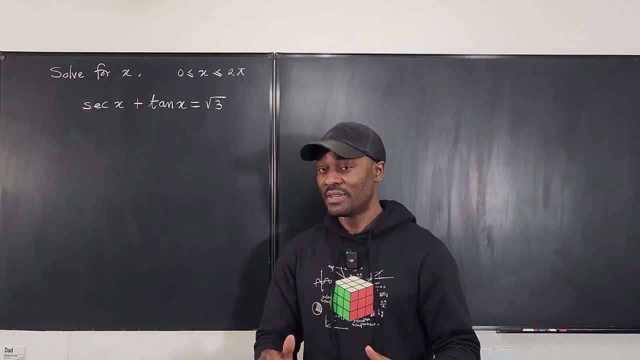 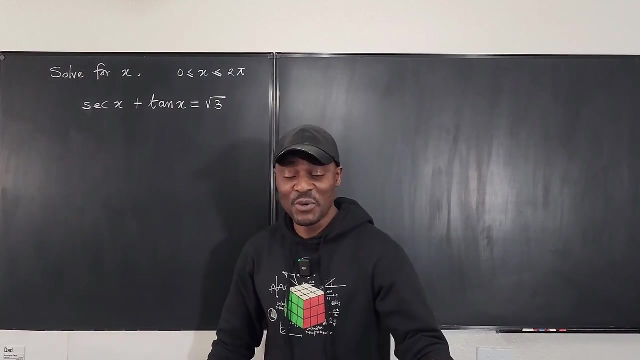 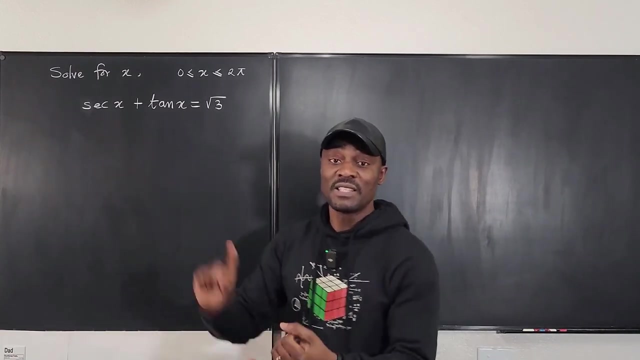 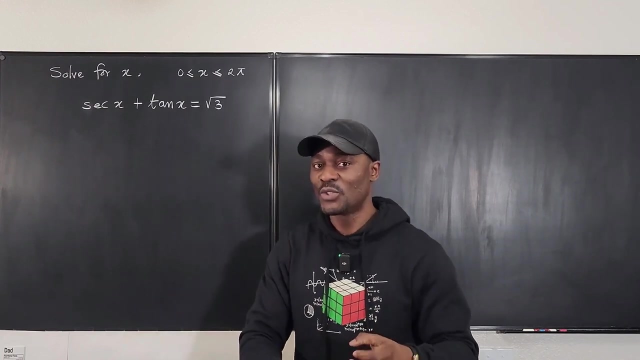 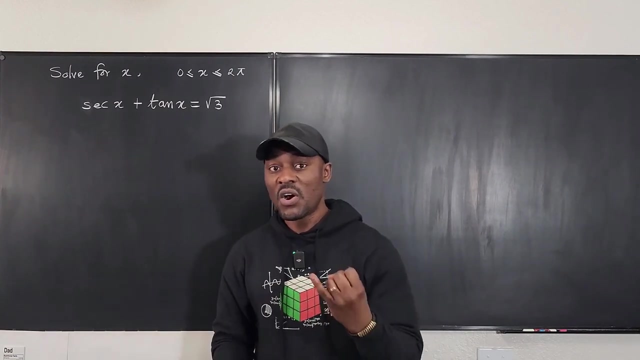 Hello, welcome to another video. We will be solving a trig equation and we have secant x plus tangent x is equal to rad 3 and we're restricting our answers to between 0 and 2 pi. So we're just doing the very first complete cycle of whatever function we're using. Well, hope it's not secant or tangent. Well, it's going to end up being sine or cosine. And how do I know it's going to end up being sine or cosine? The thing is, you really don't know how to manipulate secant. You don't know how to manipulate tangent as much as you know how to manipulate sine and cosine. So general recommendation, whenever you get a problem that is written in terms of any trig function, other than sine or cosine, I strongly recommend that you rewrite whatever the expression is or equation is in terms of just sine or cosine or both of them and then do what you want to do. 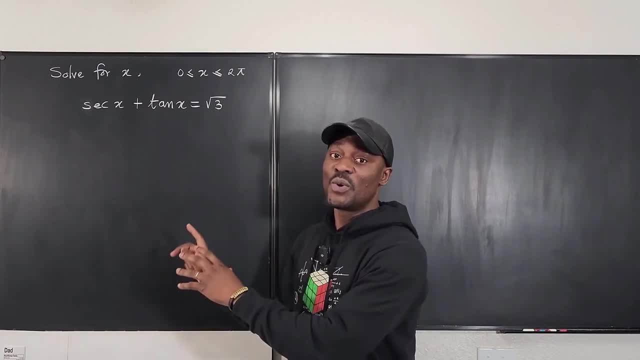 Unless it is so obvious that you know what you're doing. But right now, I don't know what I'm doing. 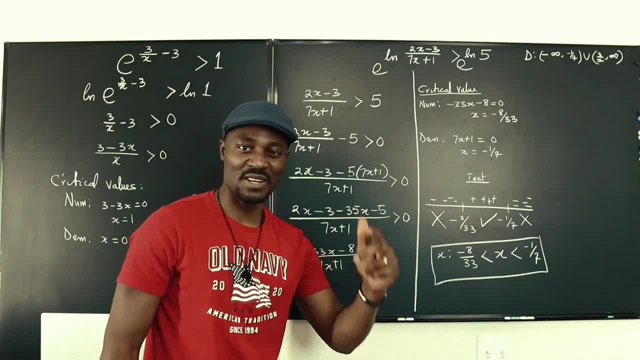 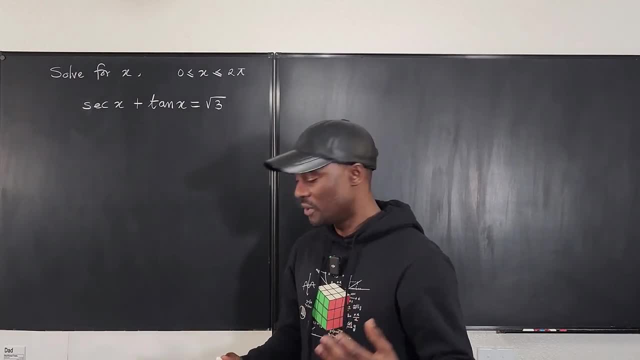 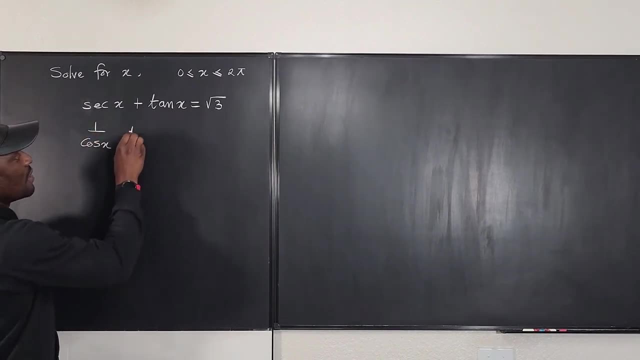 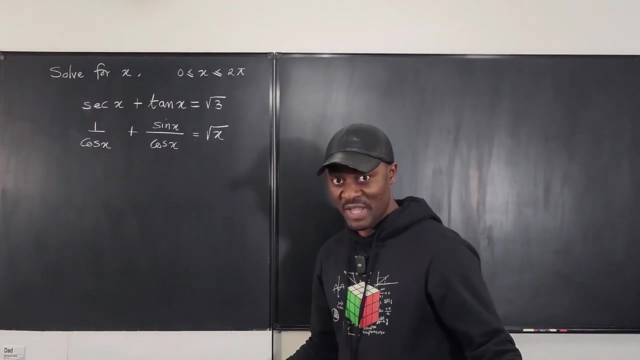 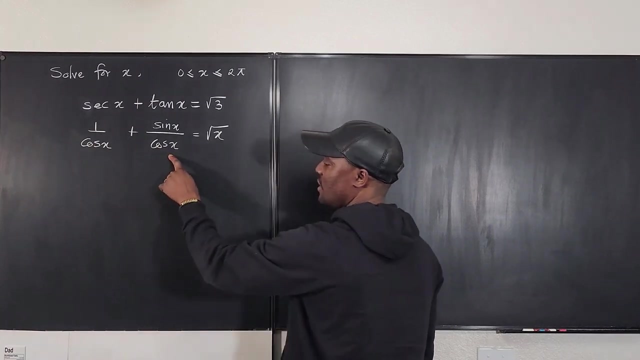 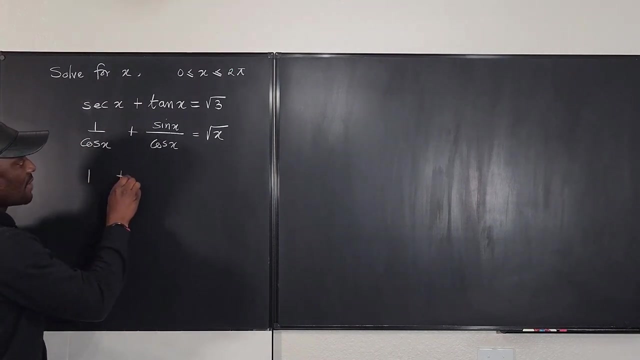 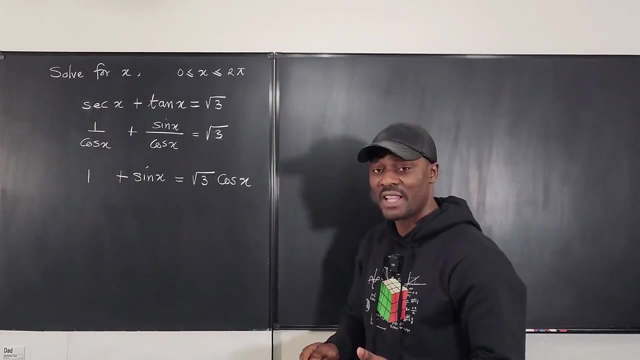 So like I said, let's change secant and tangent to what we know, sine and cosine. So we know that secant x is 1 over cosine x. And we know that tan x is sine x over cosine x. Okay. So this way now, I'm beginning to think, what can I do? Because I need to get rid of this. I need to get rid of this. I need to be able to solve it. Okay. Well, I need to get rid of all the denominators, which is usually the first thing you want to do in solving an equation. Get rid of the denominators. You don't need them. So I'm going to multiply each of these terms by the denominator that I see, which is cosine. So we're going to have, if I multiply this by cosine, I'm going to get 1. If I multiply this by cosine, I'll be left with sine x. And if I multiply this by cosine, I'll be left with the denominator. What was that? Square root of 3 cosine x. Okay. That was square root of 3, not square root of x. You have an equation now that is written in terms of sine x and cosine x. 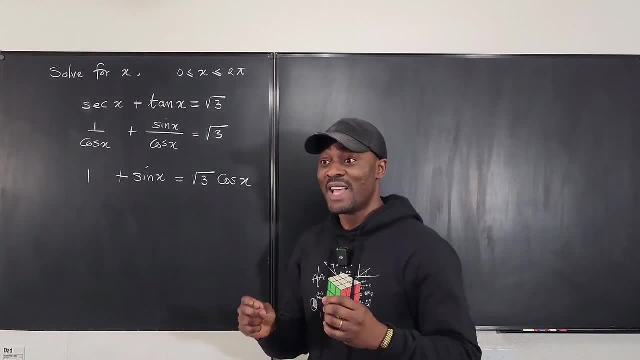 And remember, it is not easy for you to have sine x and cosine x equal each other unless you're 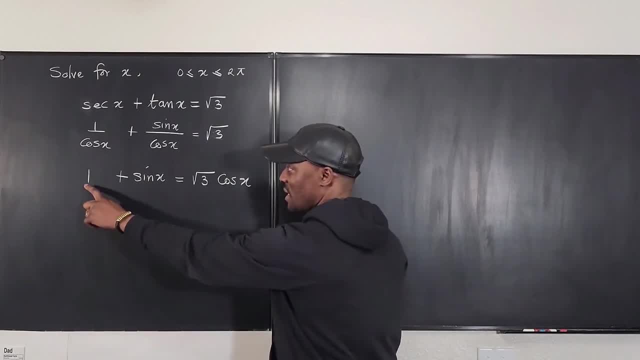 talking about the complementary angle there. But there's a 1 standing here. And that makes it very, very difficult. 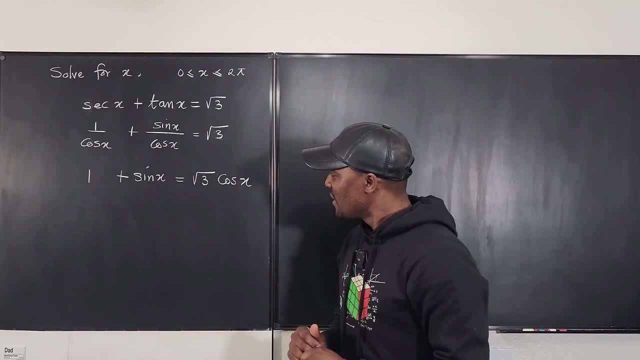 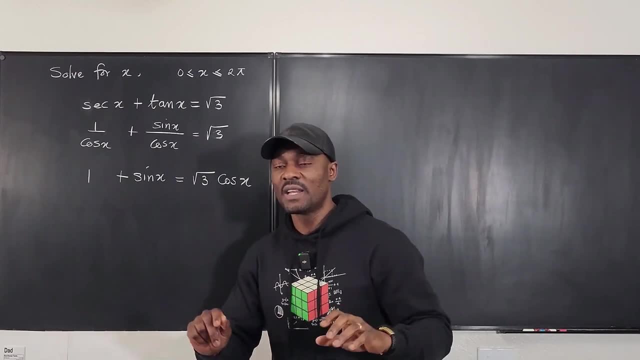 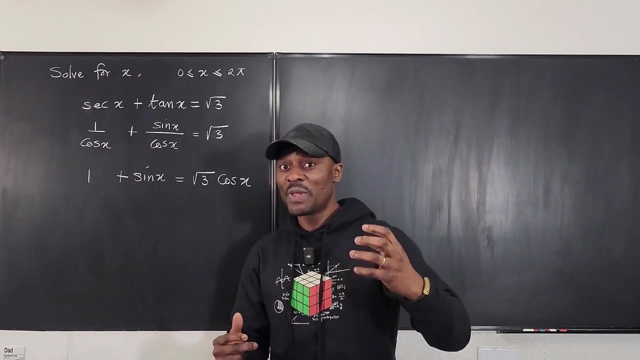 for you to do it. So what you want to do is, it's tough. So usually, whenever you have sine and cosine, you want to bring the Pythagorean identity into this. Because somehow, we know that when you 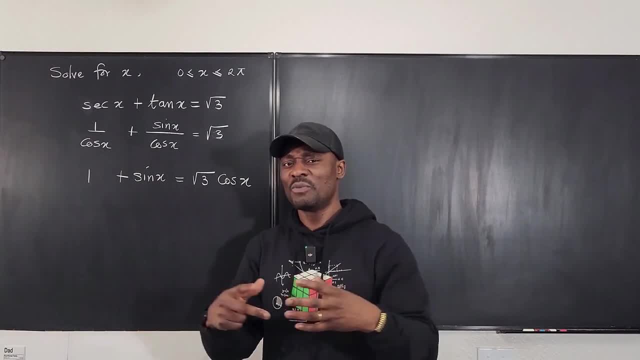 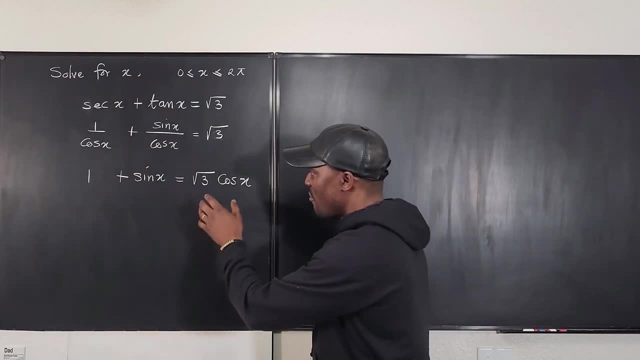 square sine and you square cosine, you can find a way to manipulate or replace or substitute the square, the squared sine or the squared cosine. So what we're going to do is, I'm going to, because 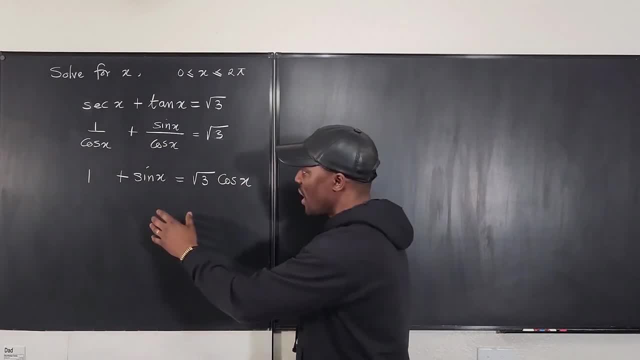 I'm trying to find, I don't see a connection. Okay. I'm going to try to square this left-hand side. And then I'm going to square this. Now, a dangerous thing you must avoid. Do not combine 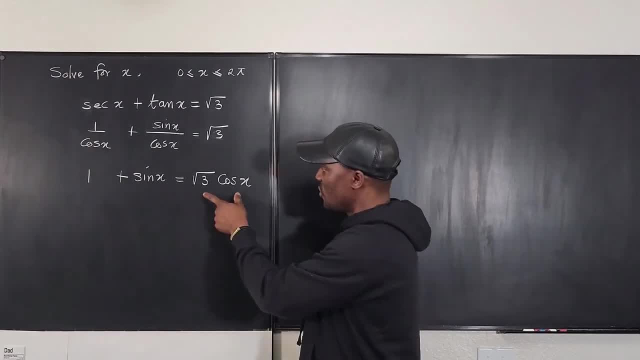 this square root with anything else. So make sure it's a single term so that when you square it, it doesn't create another radical. Because if you move this 1 here, then you're going to have 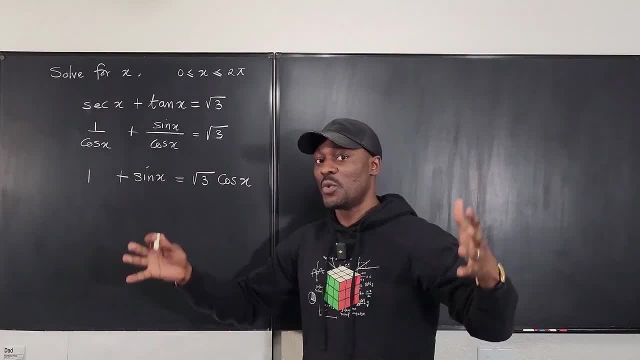 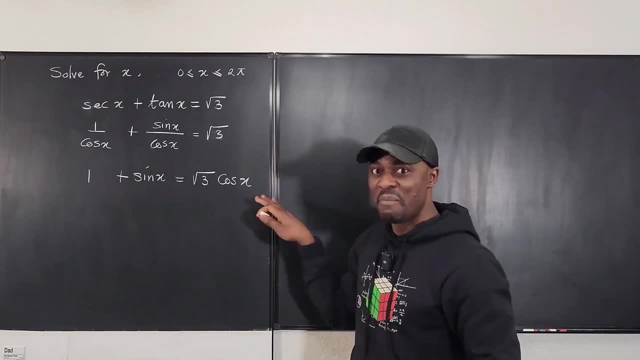 radical 3 cosine x plus 1. And by the time you square the expression, you're going to have radical, you can't use for solving your equation. So this state is the best state. Put the radical alone so 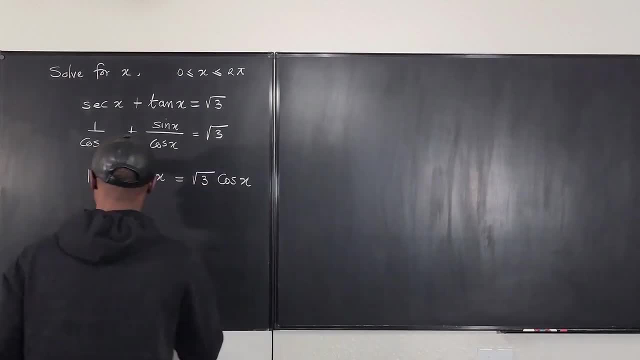 that when you square it, it just disappears. So we're going to square both sides. So we're going to square both sides. So if we square both sides, we're going to have 1 plus sine x squared will be 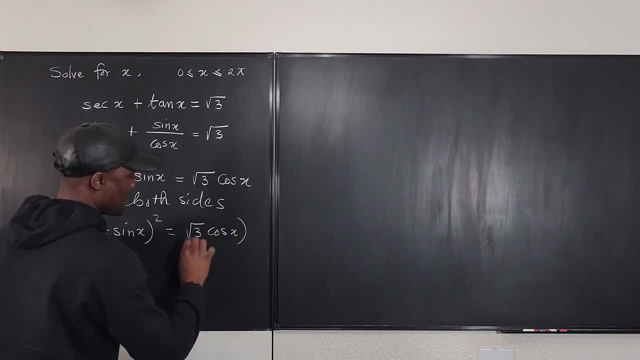 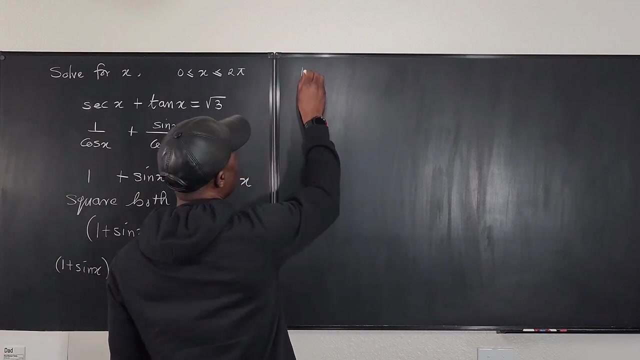 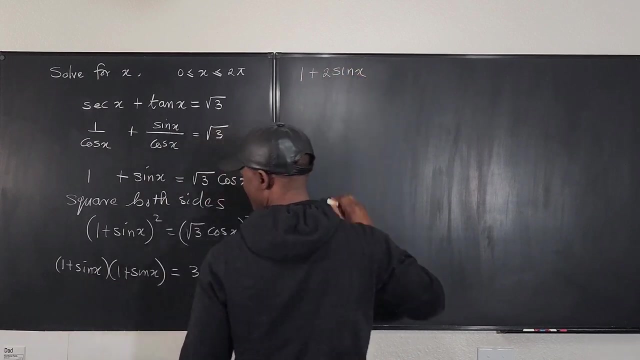 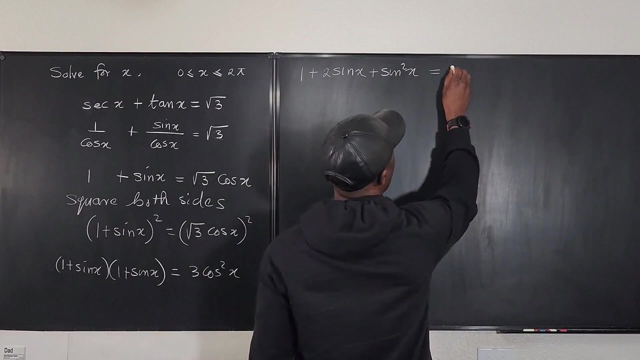 radical 3 cosine x. squared plus sine x multiplied by 1 plus sine x equals, if we square this, this is going to be 3 cosine squared x. Okay. So let's write this out. If we open this up, it's going to be 1 squared plus sine x plus sine x is going to be plus 2 sine x. And if we square this times, this is going to be 3 squared x. And on the right-hand side, we're going to have 3 cosine squared x. Okay. 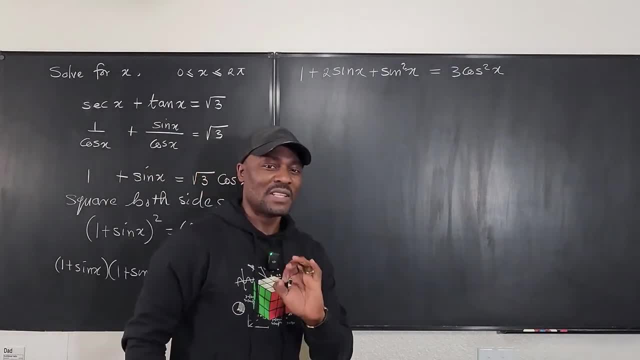 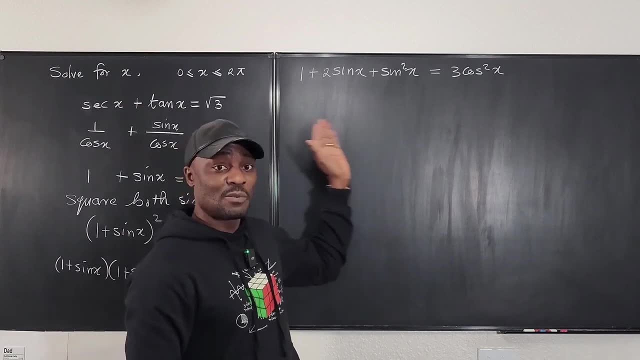 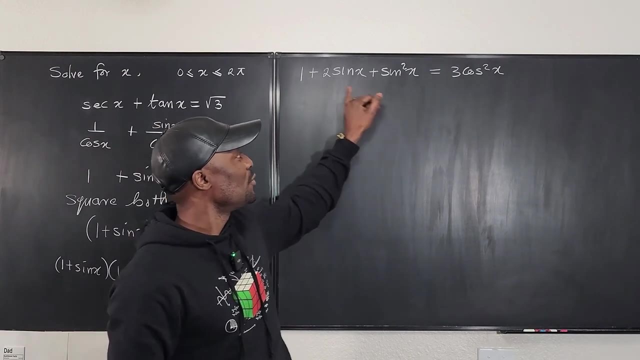 Now, this is where it becomes really, really tough. You're asking yourself, I need to convert sine to cosine, or I need to convert cosine to sine. Well, this expression makes it easy for you because you don't know how to deal with this. So you might as well look for a quadratic expression in terms of sine. 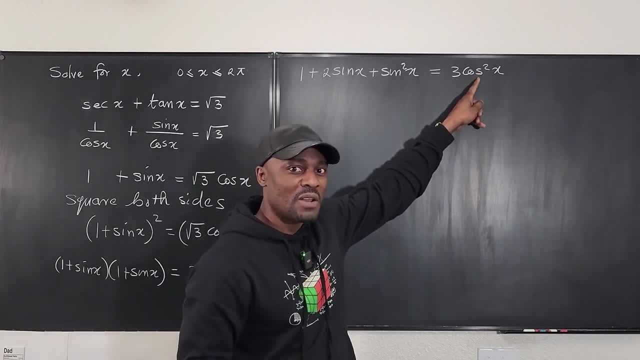 So go here and replace this cosine squared by 1 minus sine squared so that everything you have 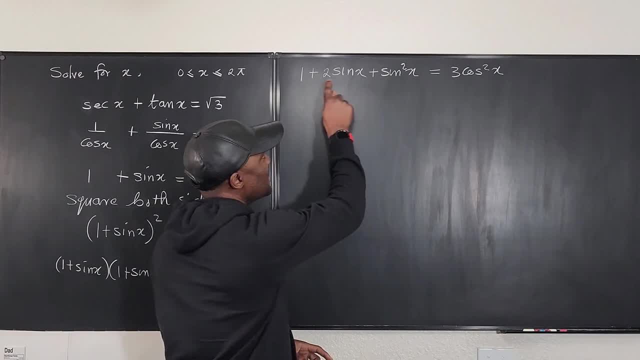 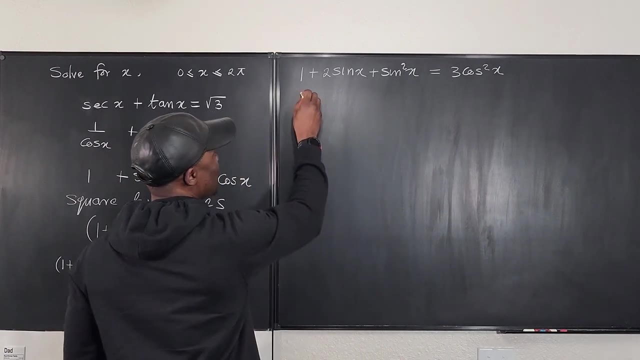 is in terms of sine. How did I decide? Because of this guy here. Because if I rewrite this as cosine, then what's going to happen is you're going to now have an equation that has sine and cosine, and you're still stuck just like the way we're stuck now. So what we've got to do is say 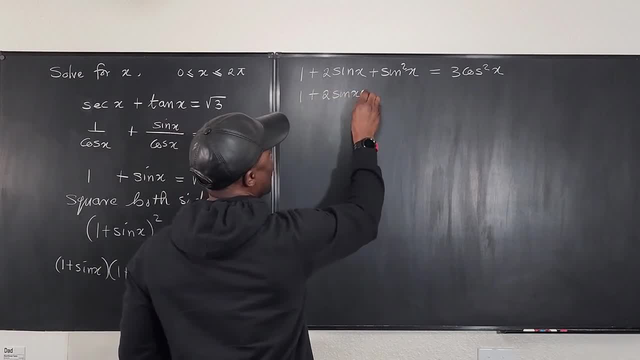 this is 1 plus 2 sine x plus sine squared x. 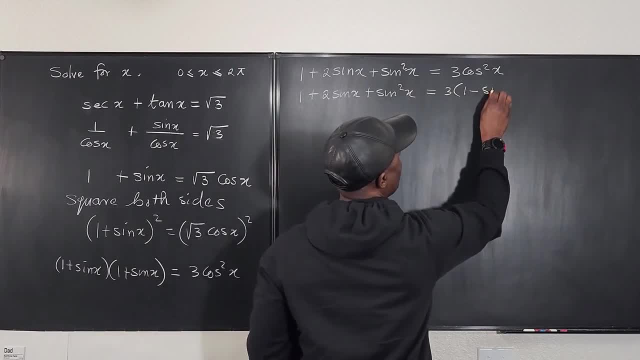 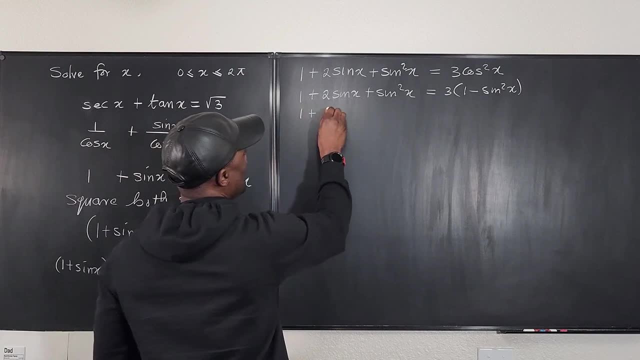 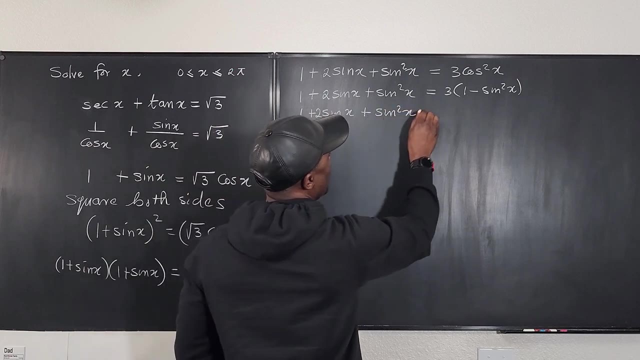 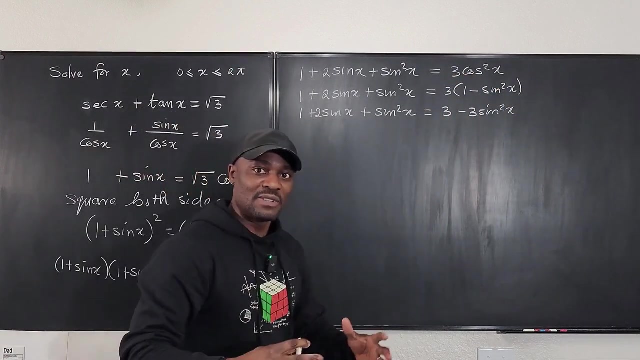 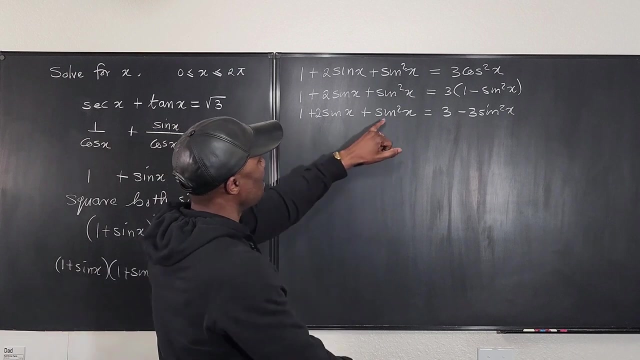 This is equal to 3 times 1 minus sine squared x. Okay. So this is the same thing as 1 plus sine x plus, sorry, 1 plus 2 sine x plus sine squared x equals 3 minus 3 sine squared x. Okay. So let's put everything together and form an equation that we can then solve as a quadratic. So here, I'm going to have sine squared x. This is 3 sine squared x. When this comes over here, it becomes 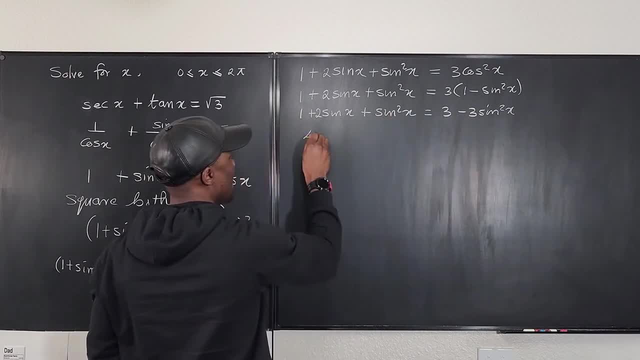 sine squared x plus 3 sine squared x. That's 4 sine squared x. 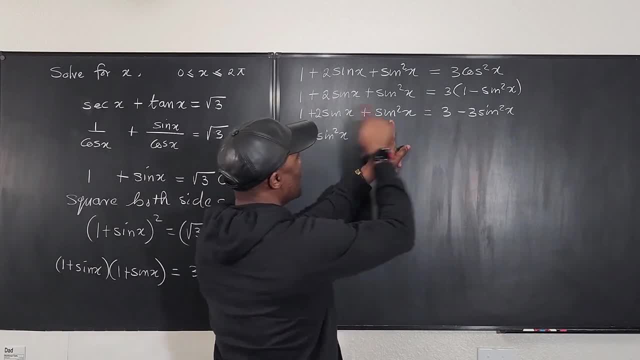 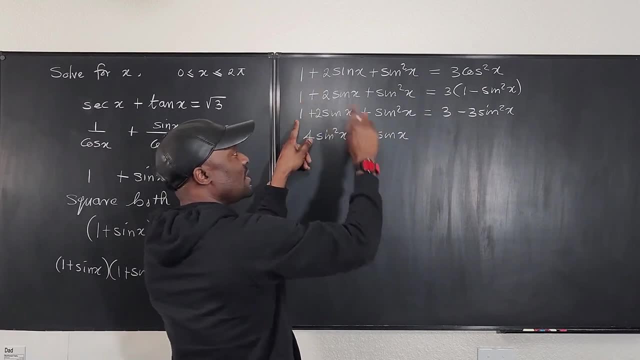 Then I look for the other term. So I've taken care of this and this. So I'm going to write this plus 2 sine x. And then I have 1. When this 3 moves over here, it's going to be 1 minus 3, which is going to be negative 2. And I have 0 here. 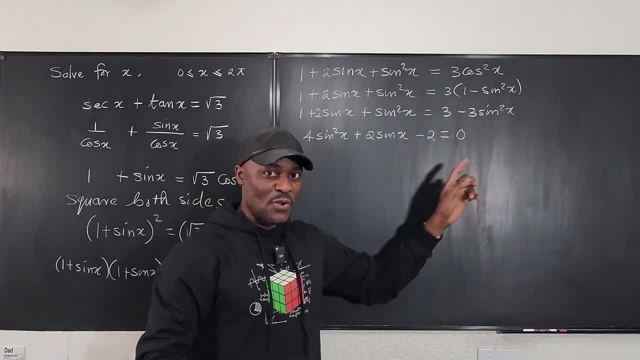 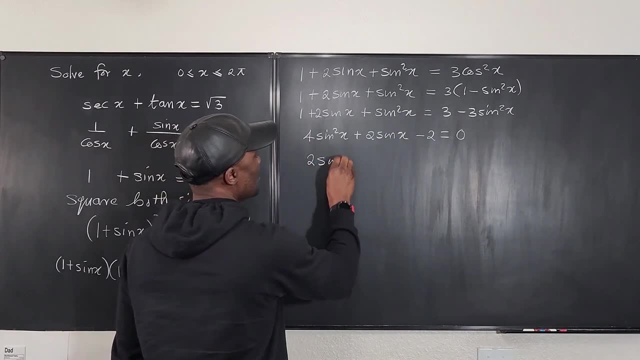 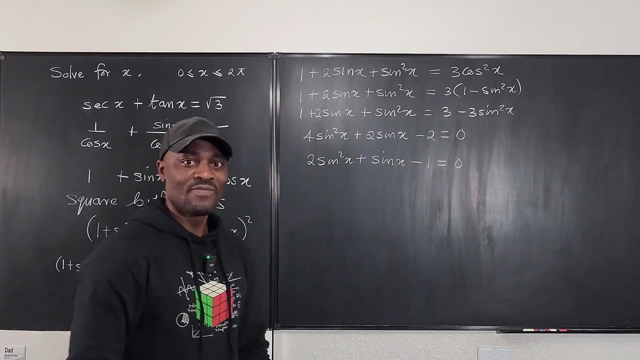 Nice. See, everything is divisible by 2. So I don't want to have big numbers I'm working with. I can divide the entire equation by 2 so that what I have left here is 2 sine squared x plus sine x minus 1 equals 0. And this looks like you having a quadratic equation 2x squared plus 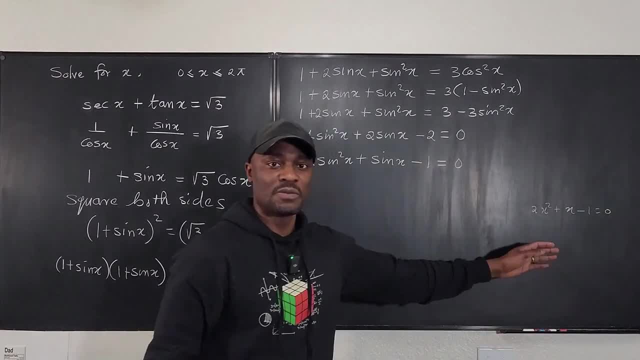 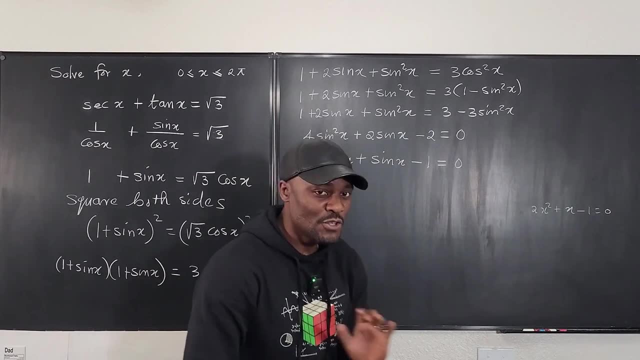 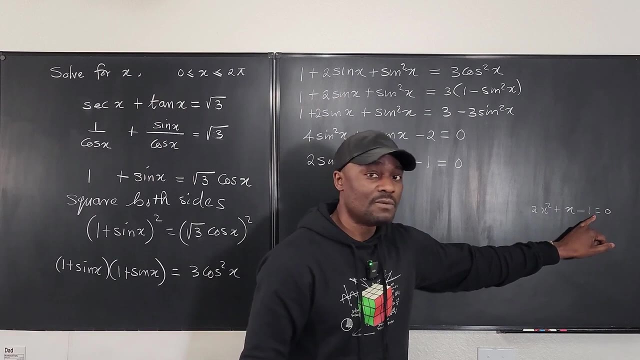 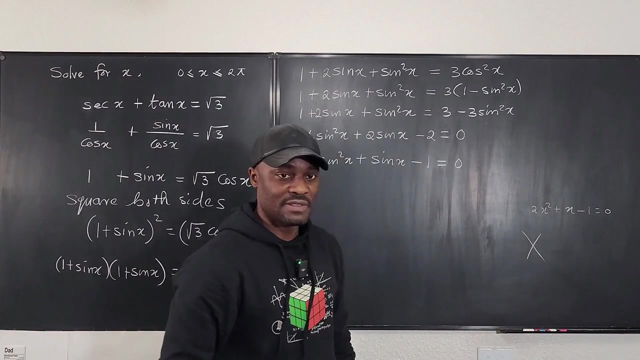 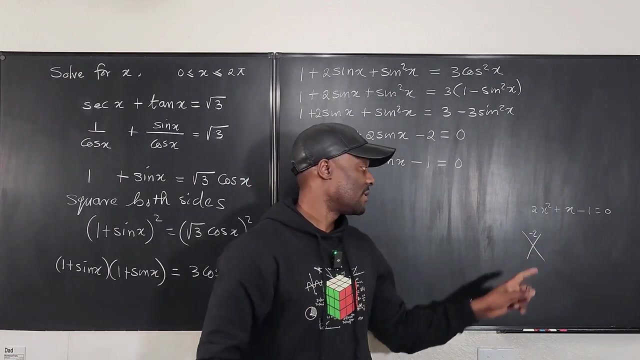 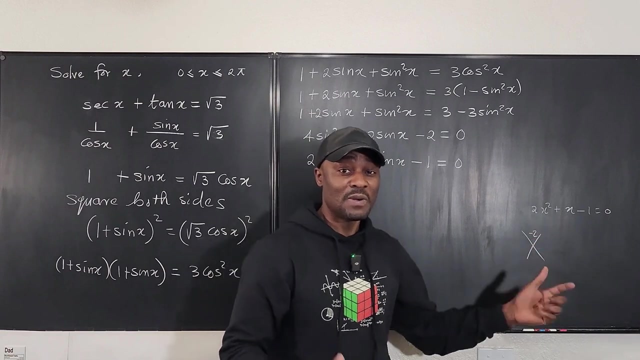 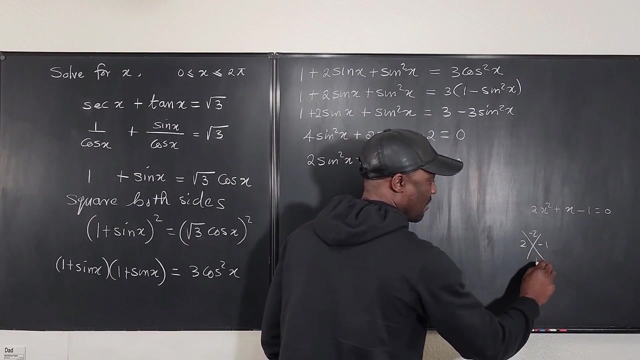 x minus 1 equals 0. How would you solve this? This can be factored. So the whole skill of factoring that you've learned, you bring it in here. How do you know you can factor it? What I'm going to do is I'm going to take this 2 and multiply the very last term. So 2 times negative 1 gives me negative 2. So I have negative 2, which is going to be on top here. Then I'm going to say I need to think of two numbers that I'll multiply together to get negative 2. But when I add the numbers together, I'm going to get positive 1. Well, those numbers must be 2 and negative 1. So it has to be 2 and negative 1 so that when you add these two together, you're going to get positive 1, 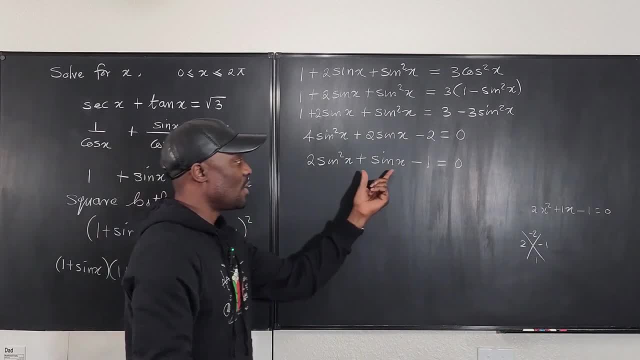 which is the number here. So that's the idea here. I'm going to go here and replace this 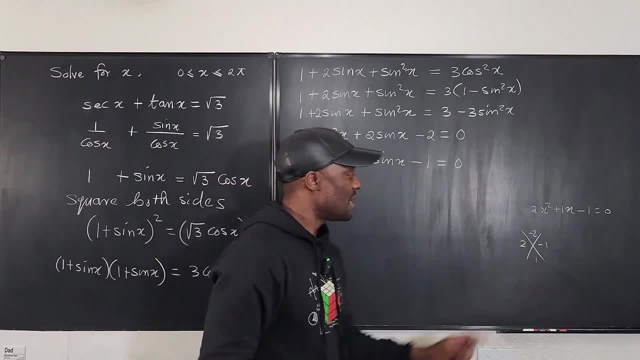 expression in the middle, the positive 1, with 2 and negative 1. So it becomes 2 sine squared x 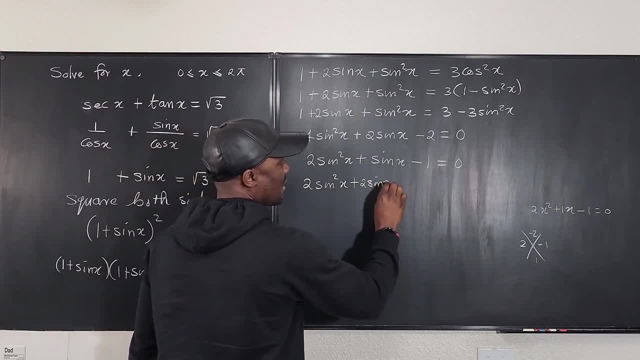 plus 2 sine x. So I've used this. Minus sine x minus 1 equals 0. So I'm going to group them together. I'll take these. 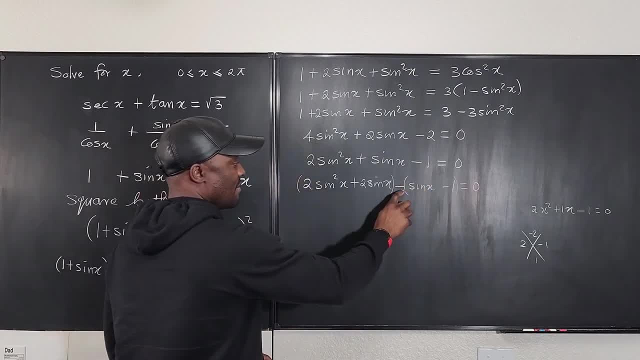 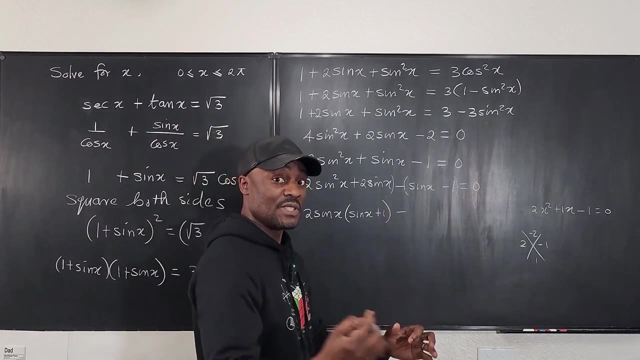 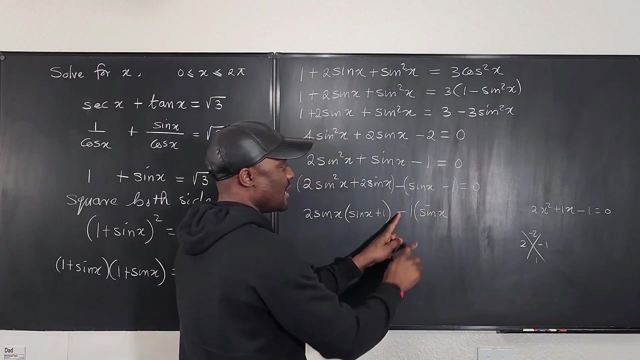 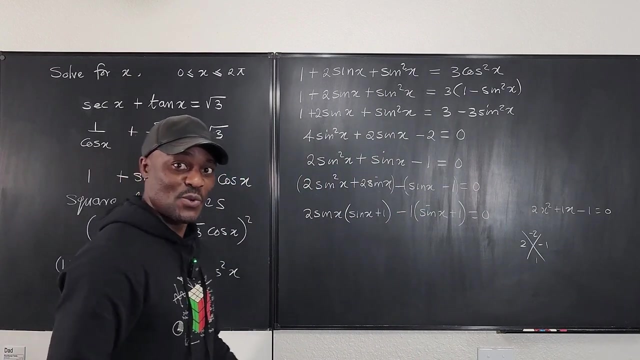 I'll take these also. Okay, leave the sine in the middle. What's common to these two? It's going to be 2 sine x. And what's left is going to be sine x plus 1 minus. What's common to these two? Nothing. So when nothing is common, you take out 1. So I'm just going to write 1 here. Okay, and then you have sine x. But this minus, if you divide this minus, it becomes a plus equals 0. So we're almost at the end of this quadratic equation because 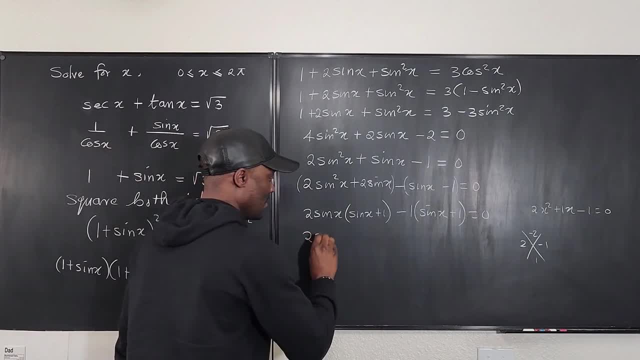 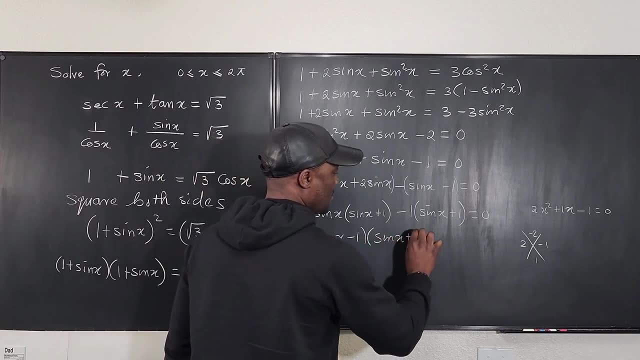 now what you have here is you have 2 sine x minus 1 and sine x plus 1 is equal to 0. 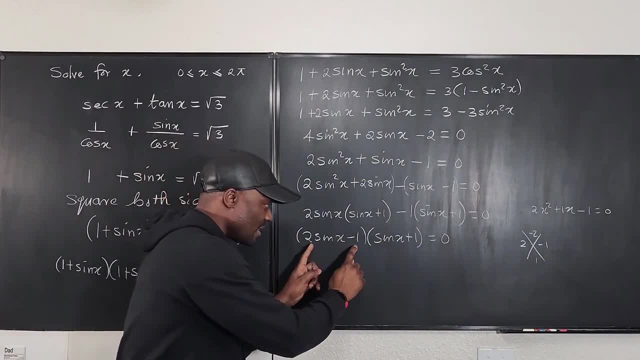 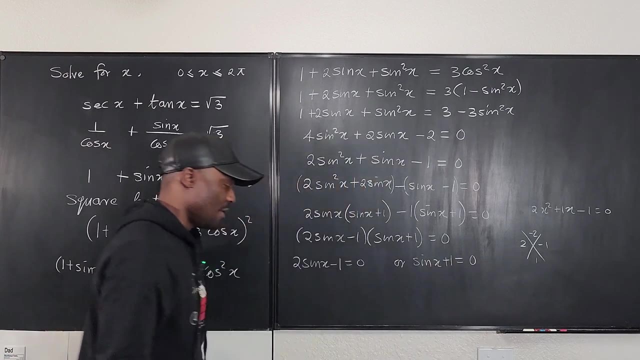 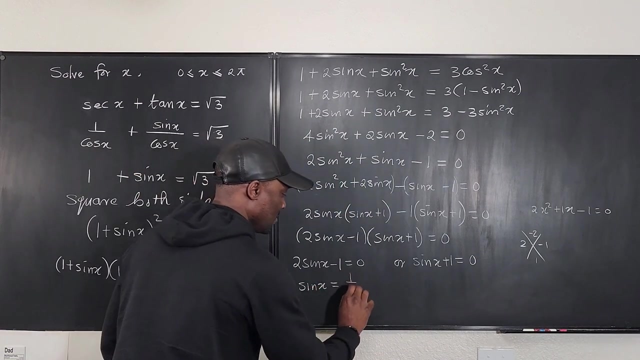 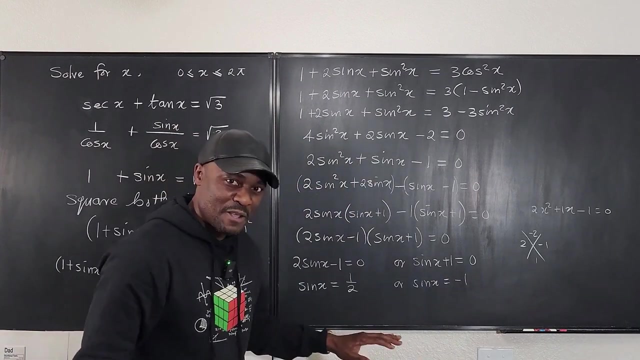 So when you have this equation like this, it means this is equal, 0 or this is equal to 0. So you're going to have 2 sine x minus 1 equals 0 or sine x plus 1 is equal to 0. And if you solve for sine x, what do you get? You get sine x is equal to 1 over 2 or sine x is equal to negative 1. So tell me, if the sine of an angle 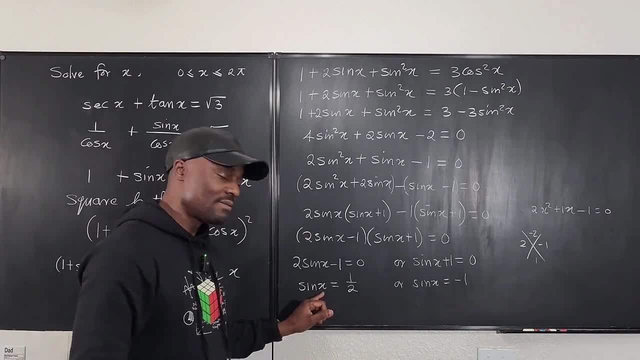 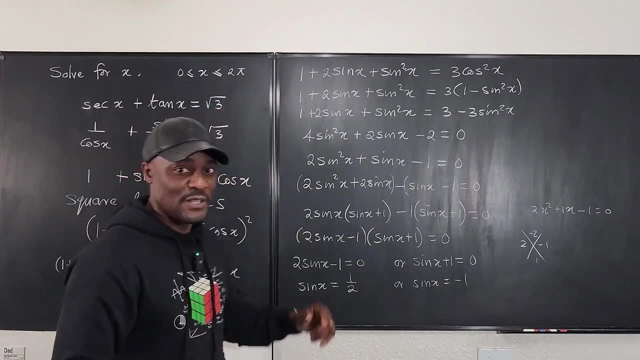 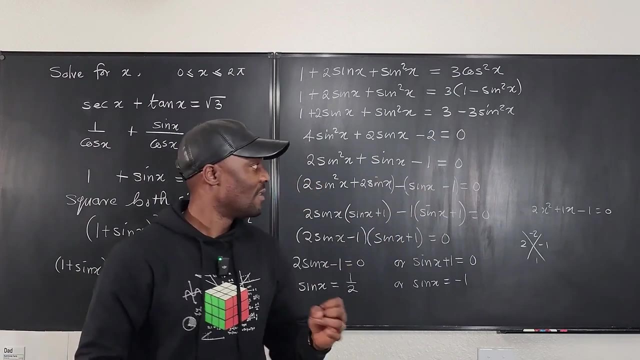 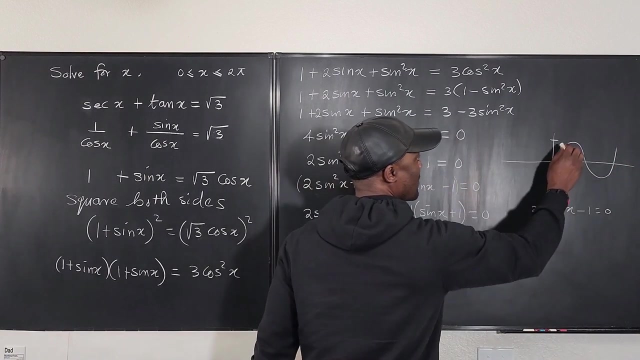 is 1 half, what is that angle? What is x? 30 degrees or pi over 6. Well, we want to find all the values between 0 and 2 pi. Well, you know that if you've memorized your unit circle or the chart, whatever you use, you know that. Okay, let's just make it easy. This is the graph of sine. We want it to be 1 half. This is 1, right? This is 1. It ends here. This is 1. So this is 1 half. Okay, so you know that for this one that has 1 half, you're going to get 2 answers. One here, one here. The first one here is at pi over 6 or 30 degrees. 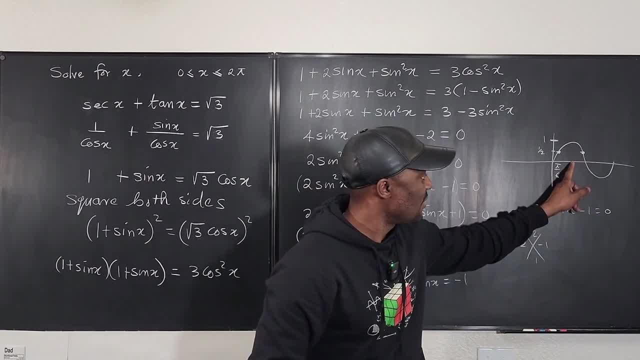 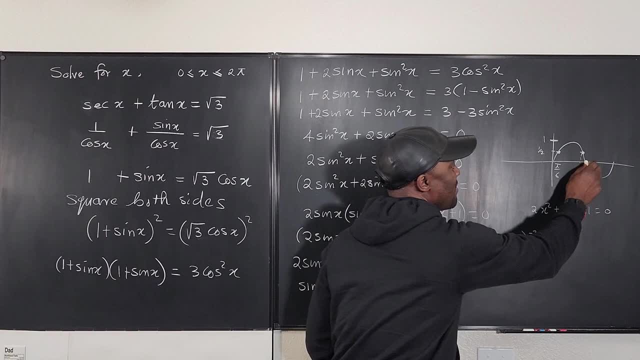 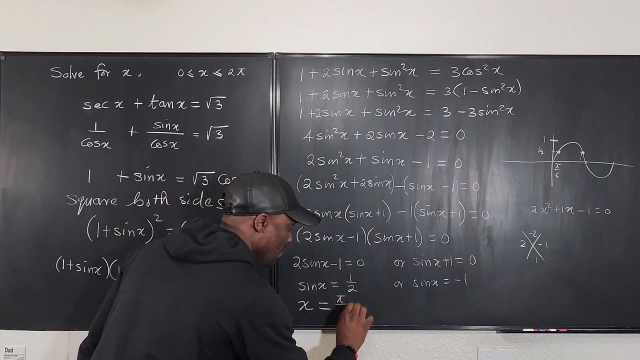 The second one here is greater than 90 degrees, but less than 180 degrees. So that would be 150 degrees because it's just pi over 6 away from this angle. So your x is going to be pi over 6. 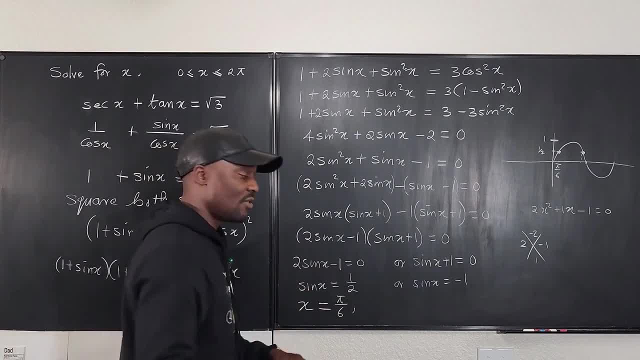 And the second possible answer is 150 degrees, which is the same thing as 5 pi over 6. 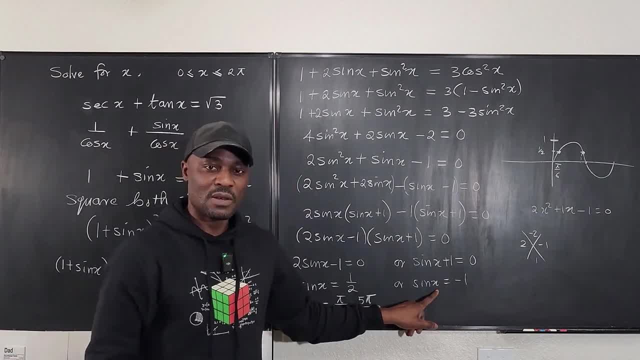 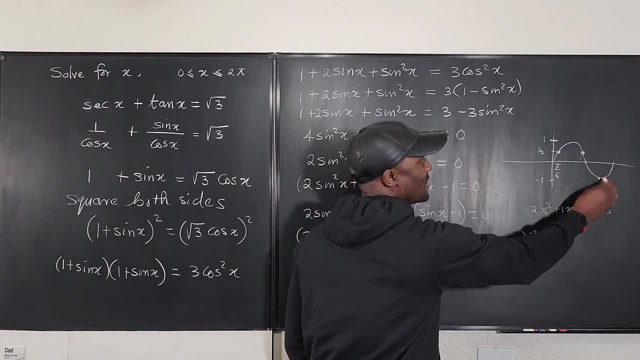 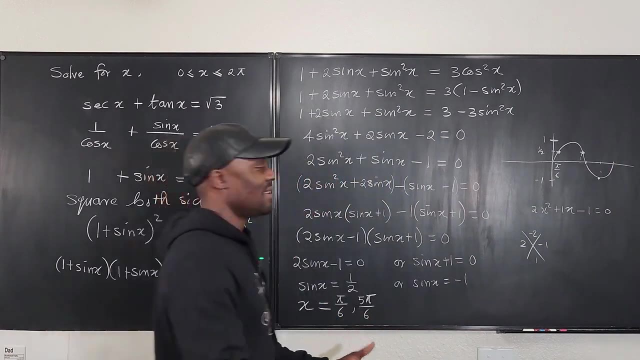 Okay. Or it could be this one. When is the sine of this angle negative 1? If you go here, the only time you're going to get negative 1 is at this point, which is at 270 degrees. Again, all these are basic things you already have memorized. Okay. And then this is going to be 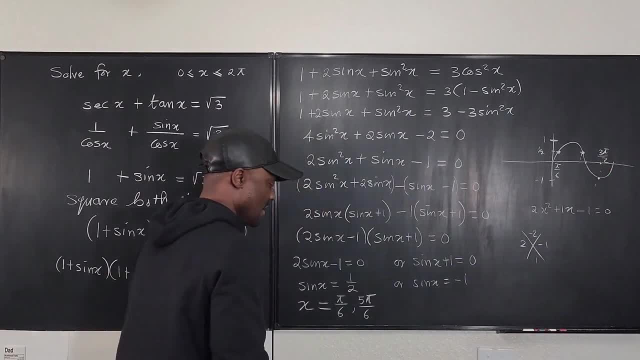 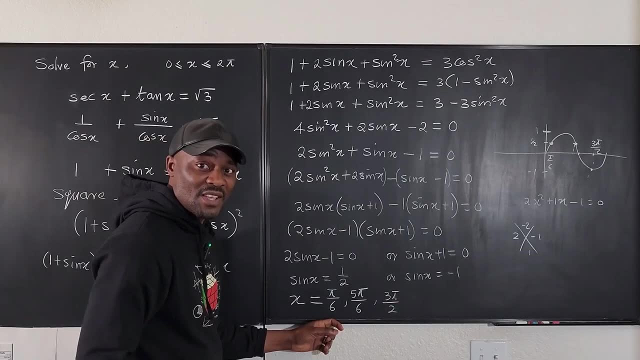 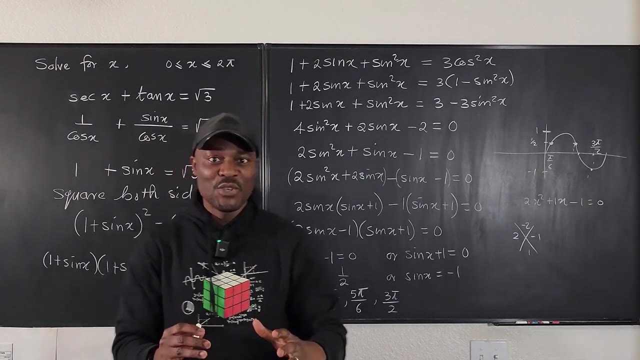 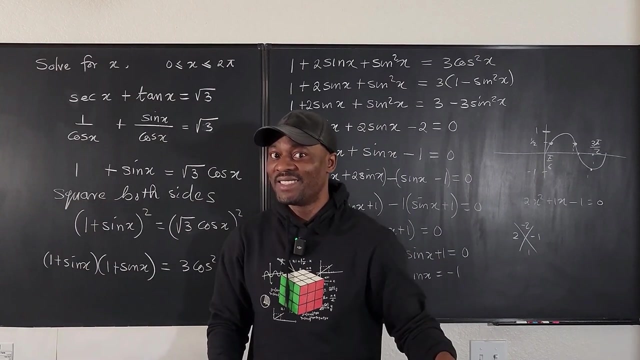 this angle, 3 pi over 2, 270 degrees, and 3 pi over 2. So the question is, are these three answers valid for the original equation? Because there's this thing about you dealing with radical signs. When you have to square both sides, you can't trust the answers that you get at the end because you've done something that's capable of removing what could have been a 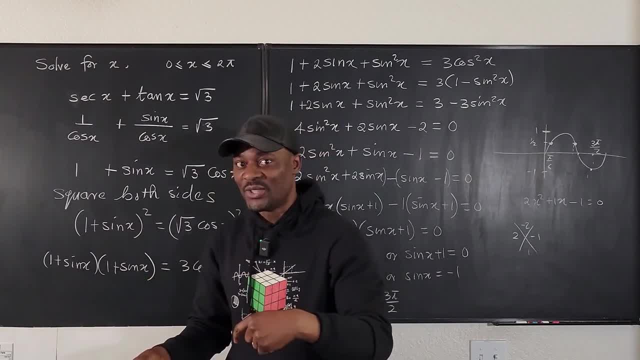 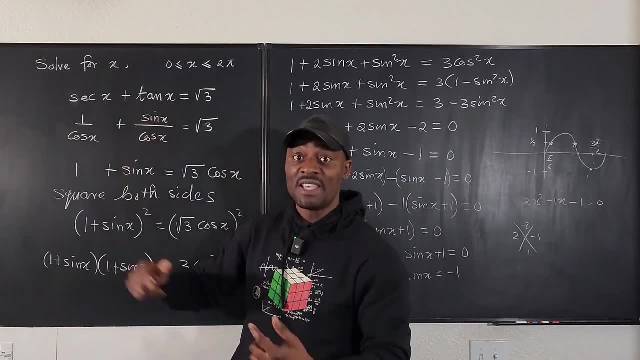 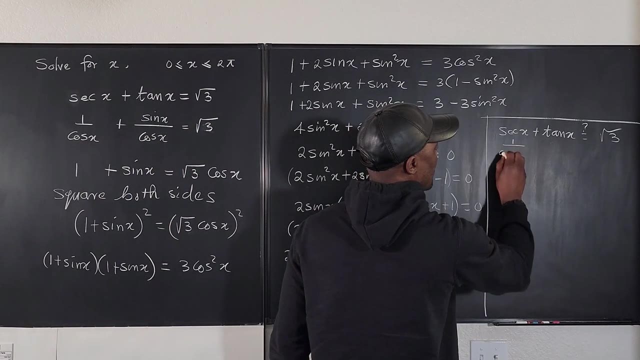 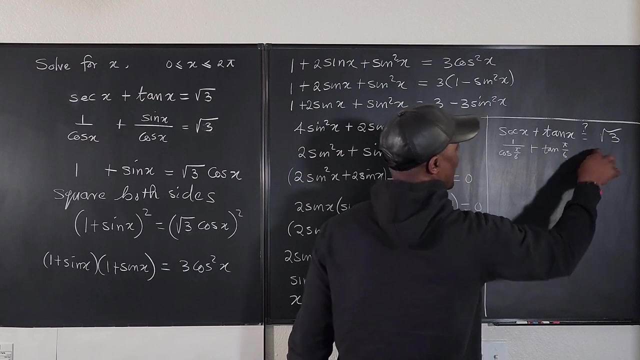 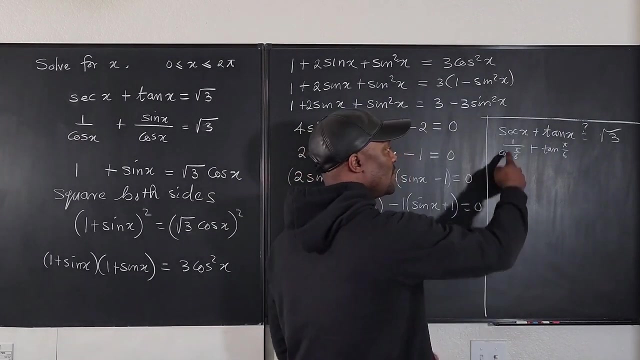 problem. So you have to go back and check what the problem was initially. So what we're going to look at is we're going to plug in each of these values into the original problem and see if it's going to give us the right-hand side. This is going to be 1 over cosine pi over 6 plus 10 pi over 6. Let's see if it's going to give us this. So we have cosine pi over 6, which is rad 3 over 2. So the reciprocal will be 2 over rad 3. And this is 1 over rad 3. We know 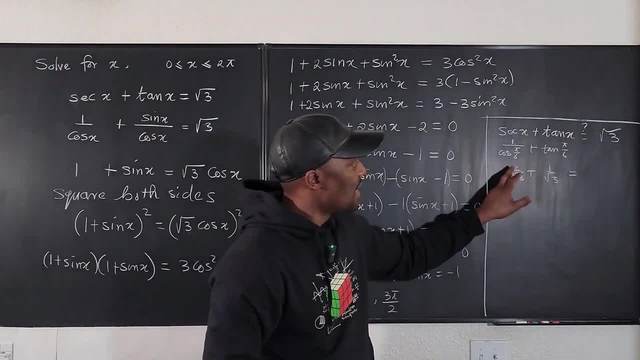 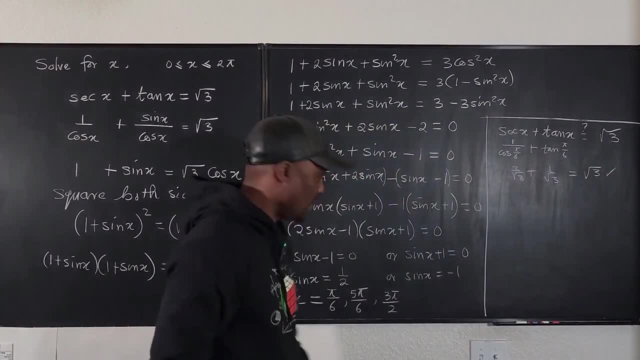 that. And if you add these two together, you're going to get 3 over rad 3, which is the same thing as rad 3 when you rationalize it. Okay. That's good. So the first value works for us. 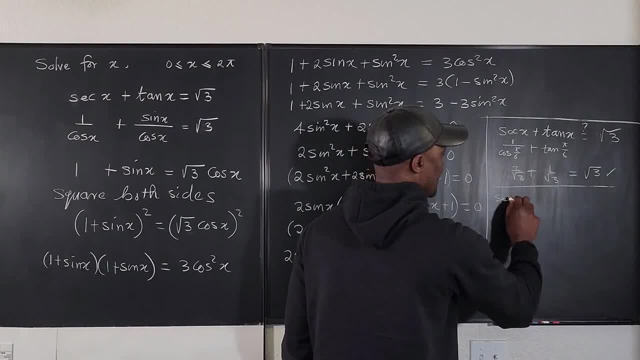 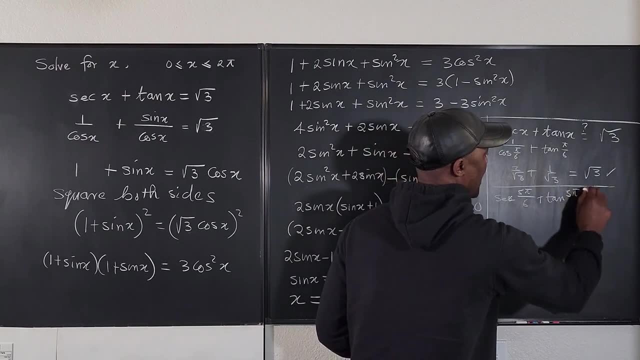 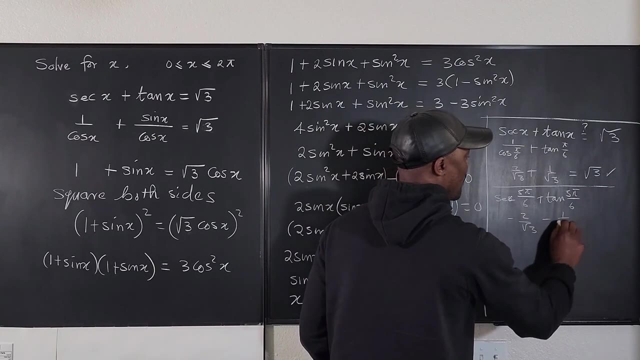 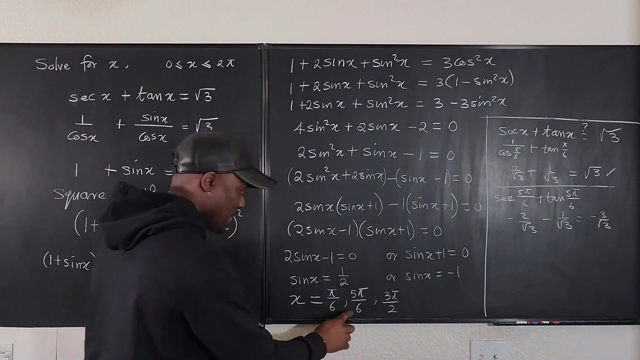 Let's go to the second one. We have secant, secant 5 pi over 6 plus 10, over 6. Well, this is going to be negative 2 over rad 3. And this is going to be negative 1 over rad 3. And that's going to give us negative 3 over rad 3, which does not give us this value. It gives us the negative version of our answer. So we can take it. So this one does not work. No.